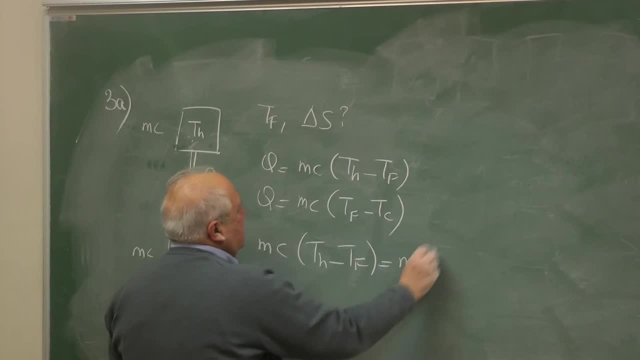 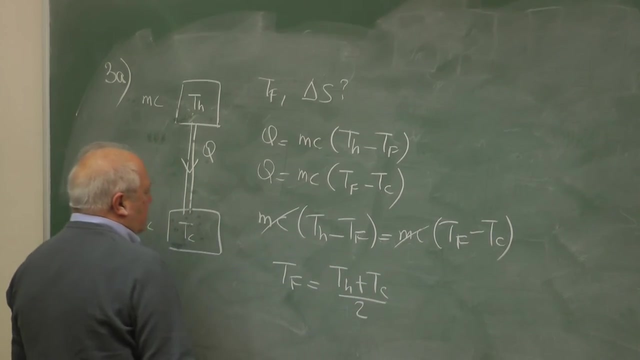 TH minus TF, that's equal to MC, TF minus TC. So MC is canceled. We see that TF is equal to: it's the arithmetic mean of these two. So when the temperature drops, of course this is because we took the two masses. 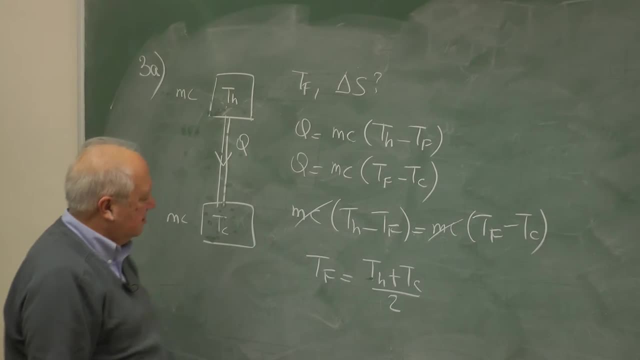 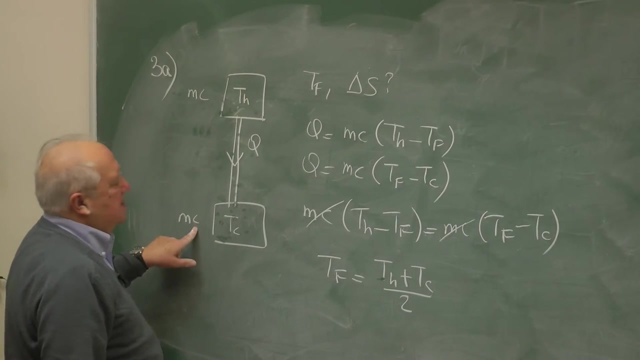 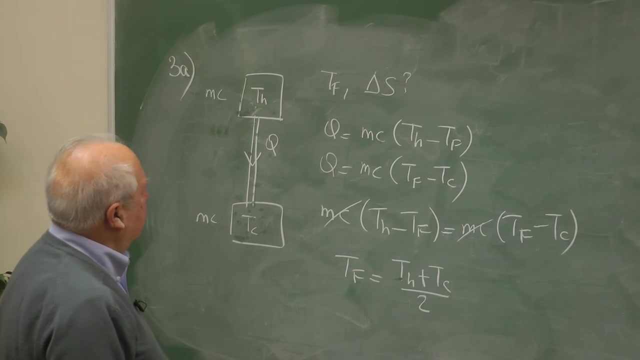 the same, Otherwise it would be a weighted average And the same. we took the same specific heat, just to keep all the algebra simple. So this is the final temperature. What about the entropy? This has lost Q at temperature here. 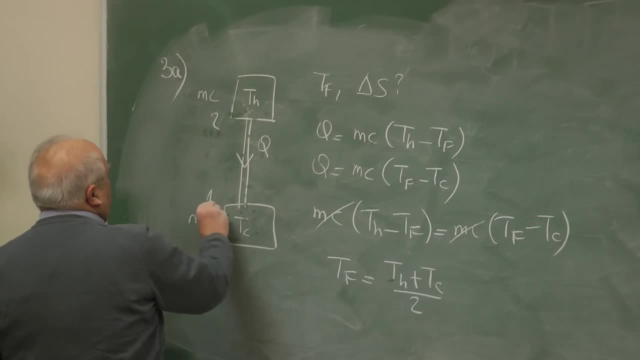 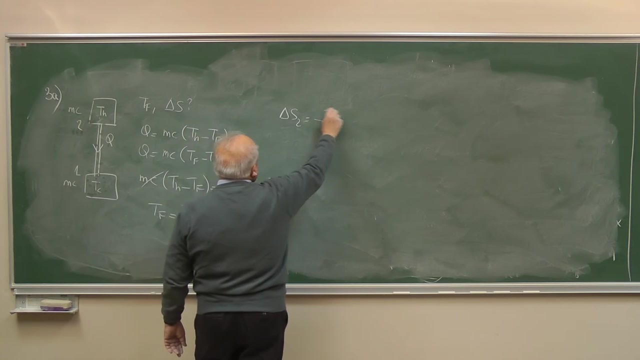 So let's call it, let's say 2 and 1.. Delta S2 is minus T. yes, We have to undo this. The heat involved is MC DT. We divide, this is the delta Q, We divide by T and integrate from the initial to final. initial to final. 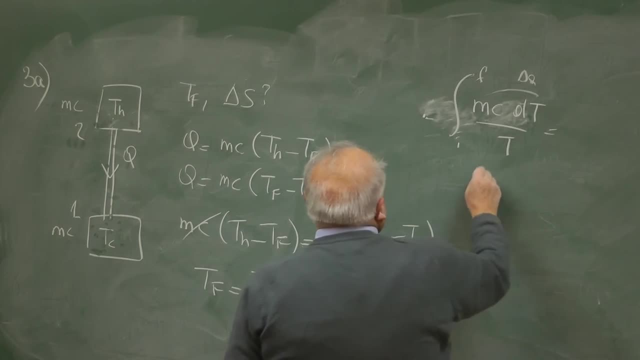 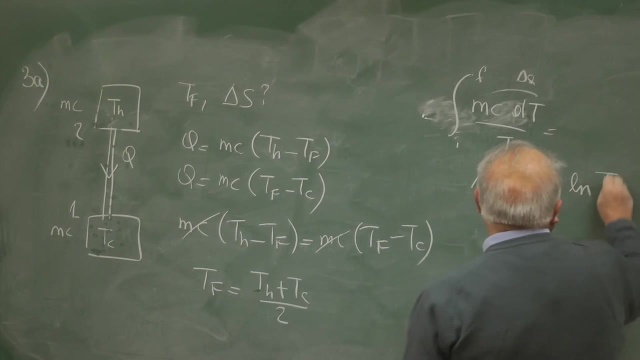 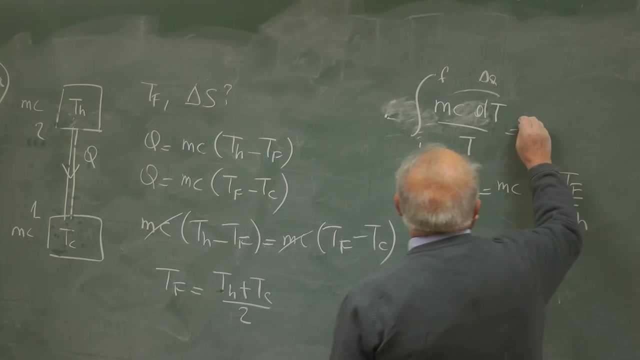 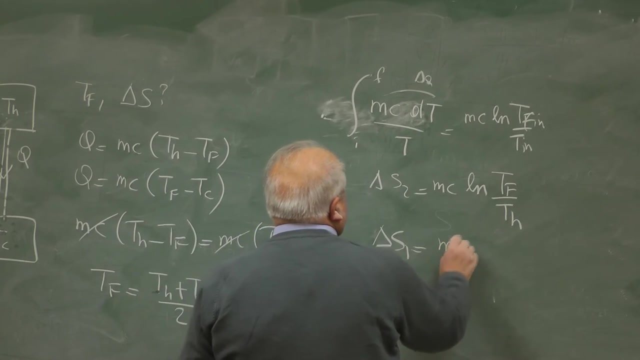 That means delta S2 is equal to MC log. the final temperature is TF. Initial temperature is E TH. This is MC log TF over T final over T initial for both of them. So delta S1 is the same MC log TF over T C. 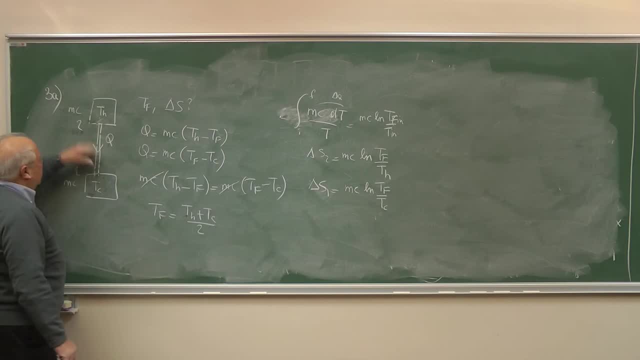 Again, although this process is irreversible. heat rushes and finally equilibrium is reached, But we are calculating. it is as if we have done it reversibly, because otherwise we cannot compute the entropy. Why can we do it? Because entropy is a state function. 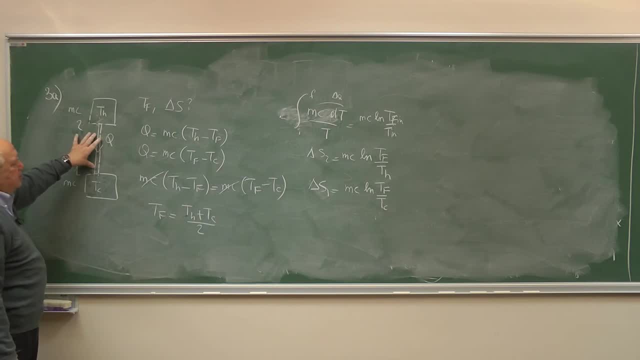 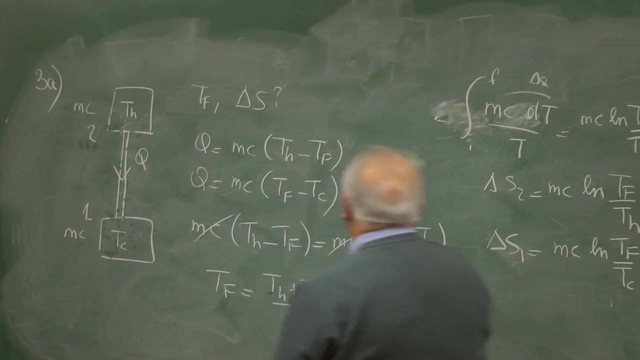 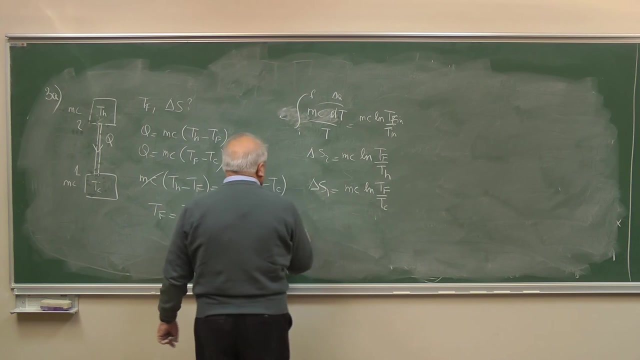 Even though this process was irreversible. we are computing the entropy change through a reversible process, As if heat did not rush, but we have reduced the temperature of this thing slowly, All right. So delta S1 plus T, S1 plus S2 is equal to MC log TF squared over TH times T C. 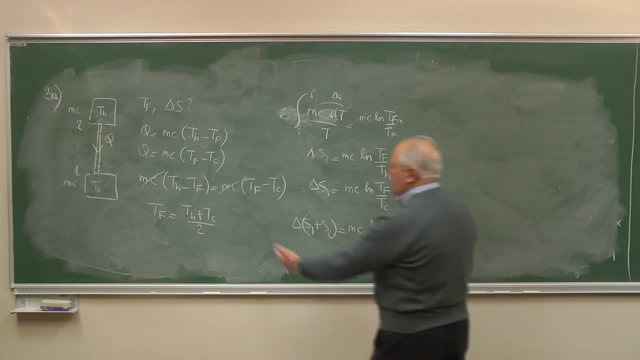 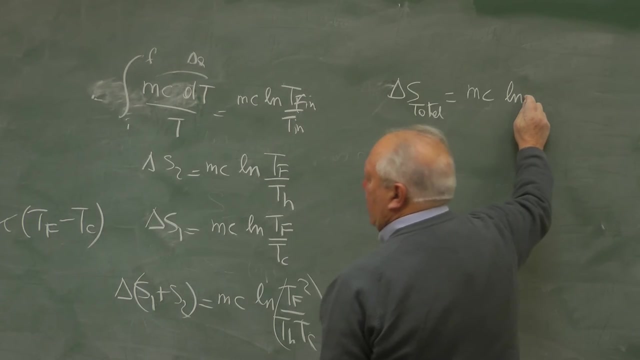 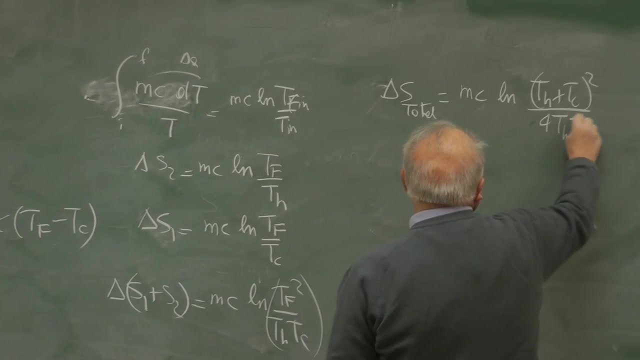 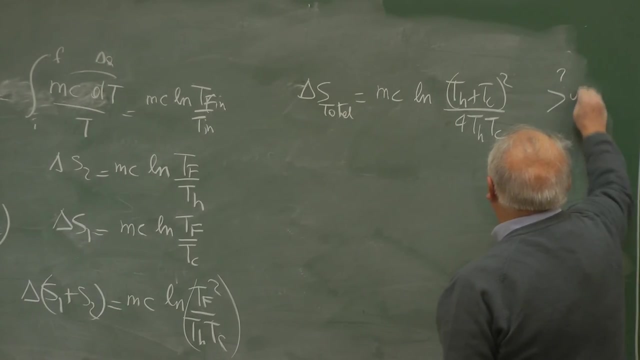 But we found what TF was. It is the arithmetic mean. So delta S total is equal to MC log TH plus T C, squared over 4 TH T C. Now the question is: is this larger than 0? Did the entropy increase? 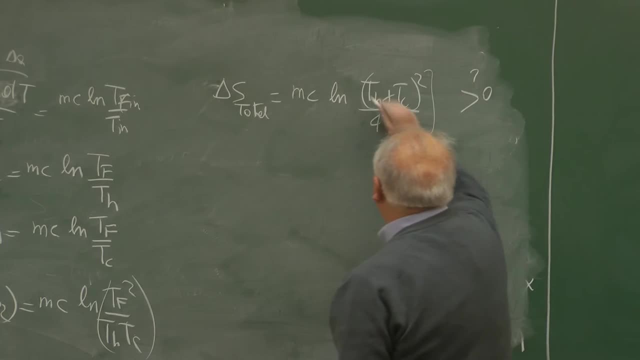 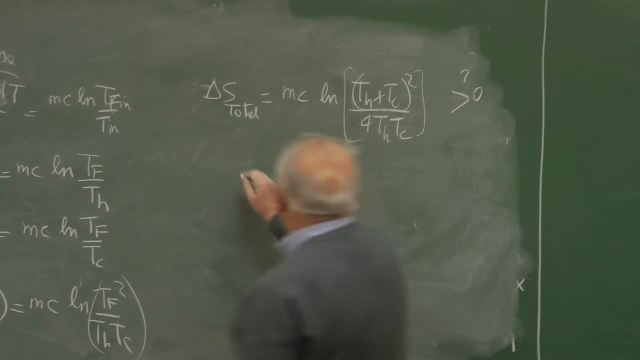 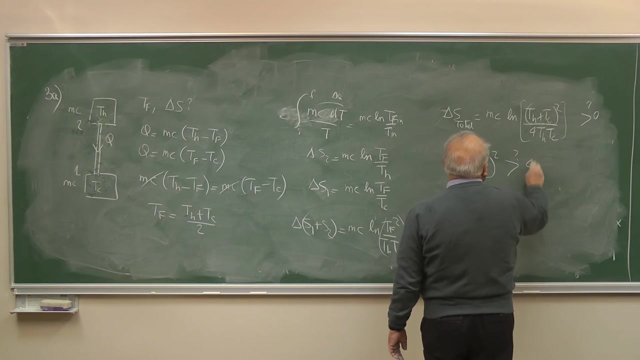 That means the logarithm argument has to be larger than 1.. Otherwise log is negative. So let's check. that Is TH plus T C squared. is it larger than 4 TH- T- C? We bring it to the left side. This will have all right. let me just do it. 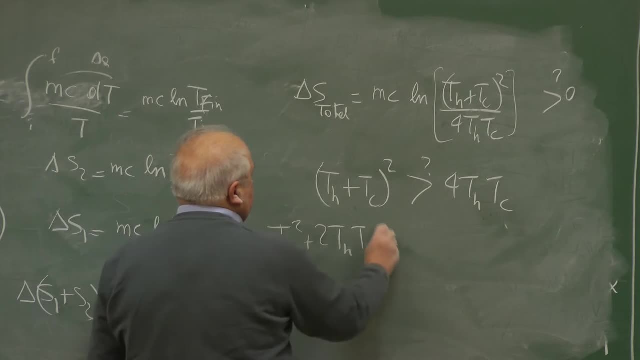 TH squared plus 2 TH T C plus T C, squared minus 4 TH T C. So this knocks it out minus 2.. Now you see that this is TH minus T C squared. Since hot temperature was larger than cold temperature. this definitely. 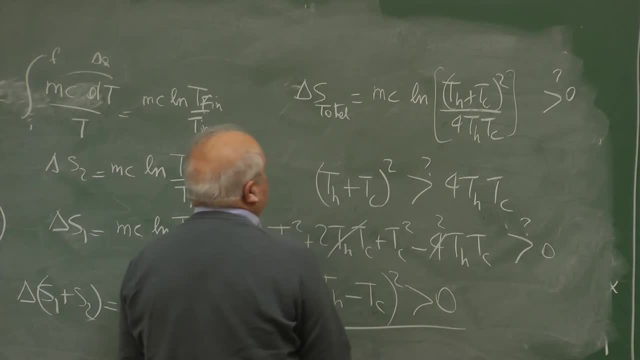 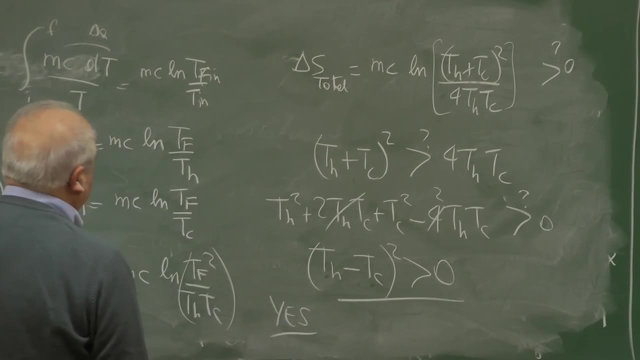 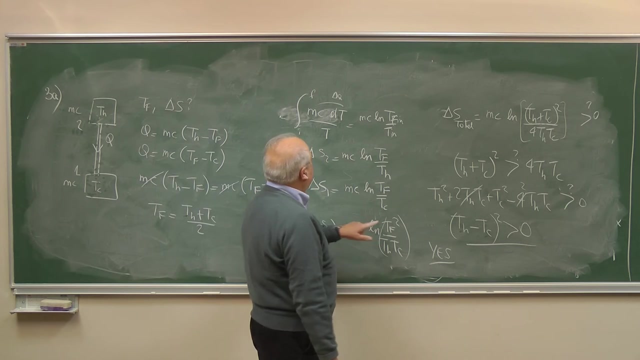 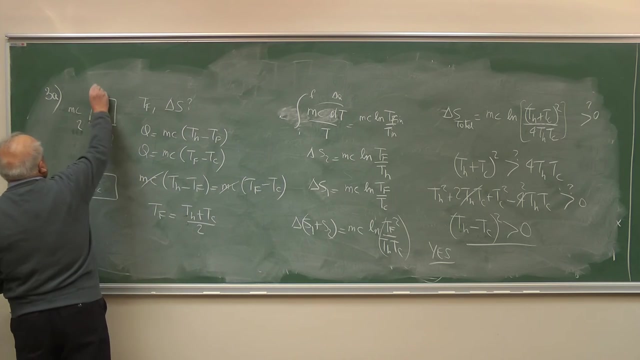 and we are taking the square, this is larger than 0.. And the answer to that is yes, It has increased by this amount And it was an increase, with TF being the arithmetic mean of these temperatures. This is the part 1 of 3A. 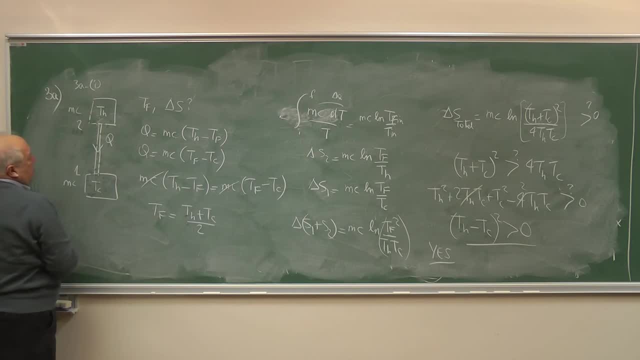 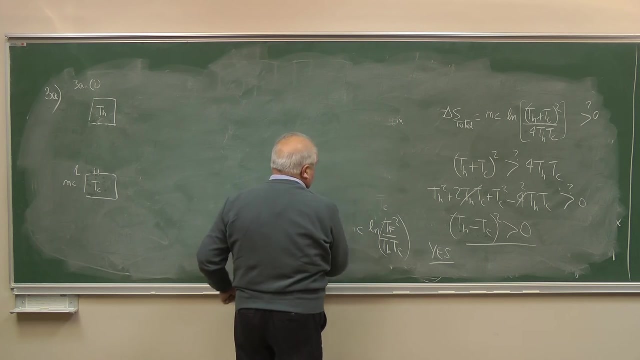 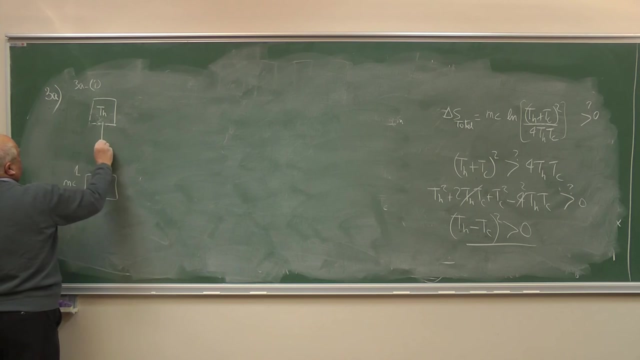 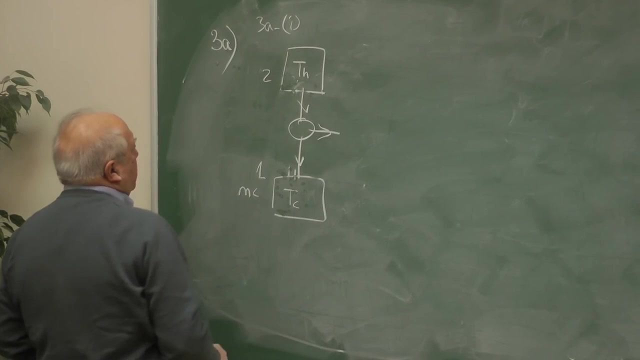 So this is 3A, part 1.. Part 2, we will operate a reversible engine. So this line here is 1A. Let us cut a number here to 2.. This is 4A. So once it is at 4A, this Pennsylvania has a power at кого. 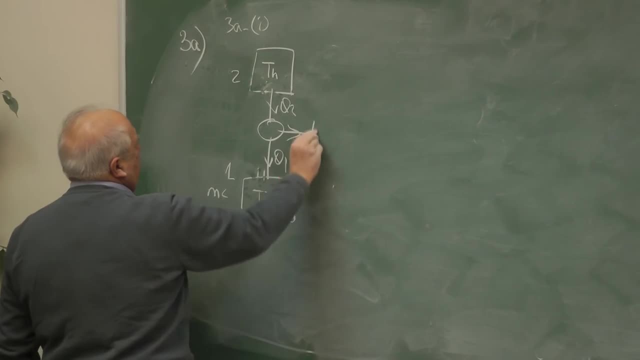 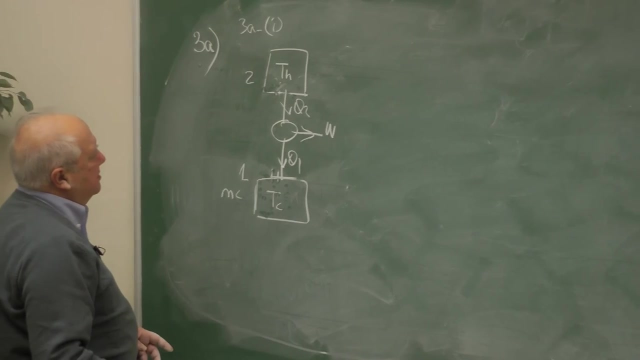 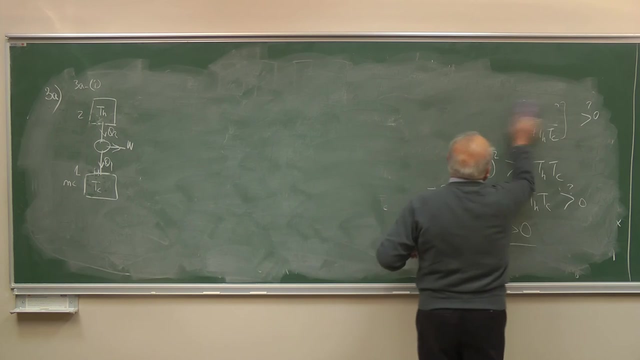 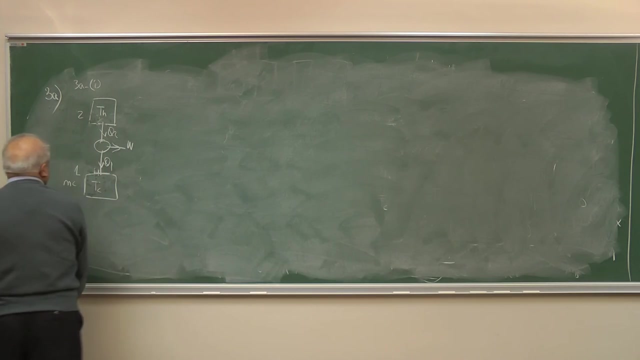 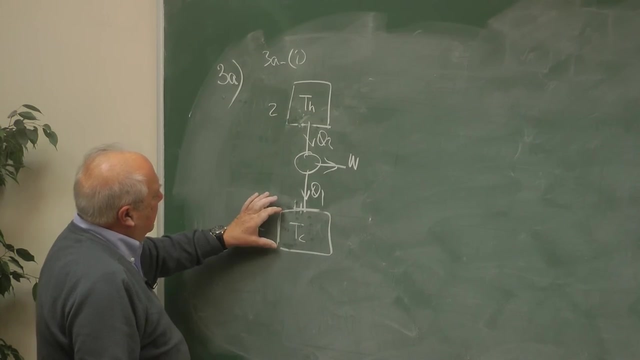 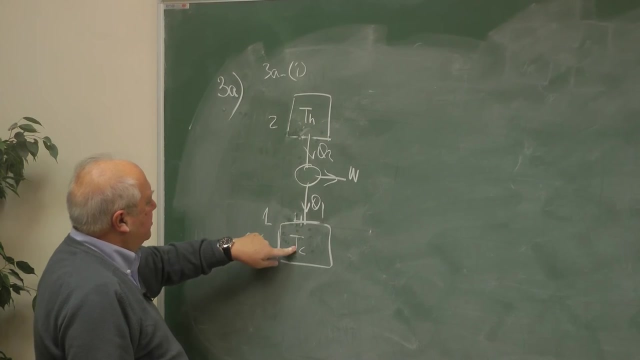 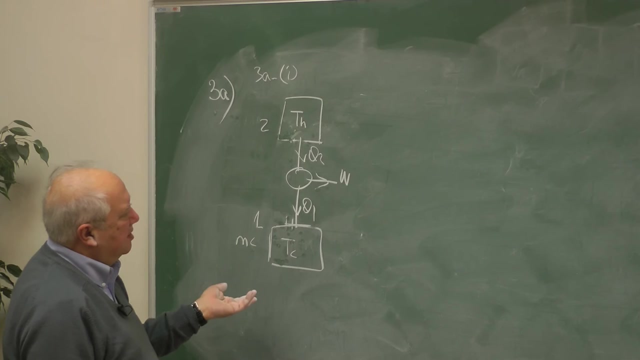 3A See. So again this part also. again, we assume these cycles are infinitesimal, namely every cycle temperatures of these blocks change a little etc. But at the end Q2 amount of heat is taken from TH and Q1 amount is dumped onto lower reservoir and W work was done, If the engine is. 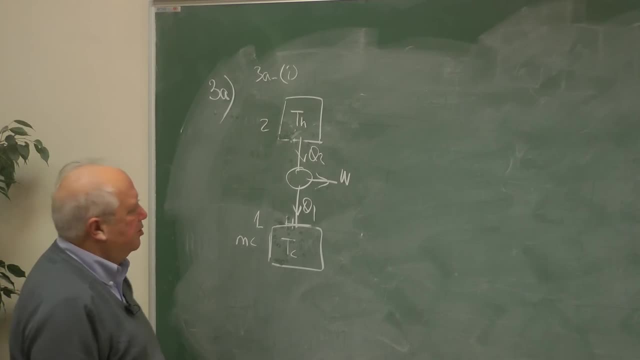 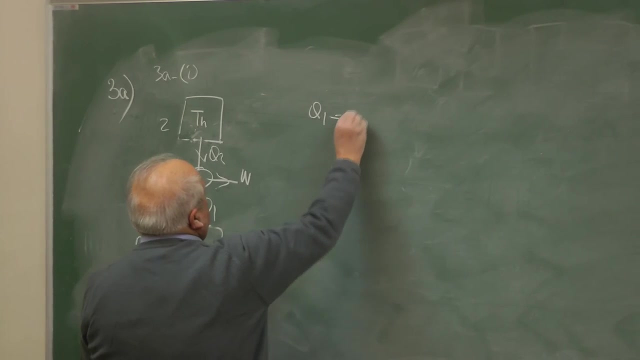 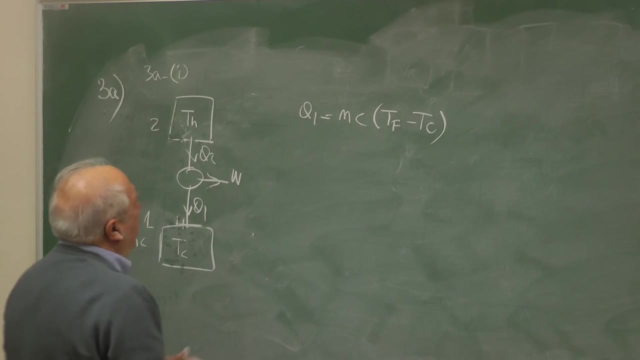 reversible and of course, this provides the maximum amount of work. So Q1.. Q1 is equal to MC TH minus TC And Q2, the heat given off is MC TH minus TF and Q2 is equal to Q1. 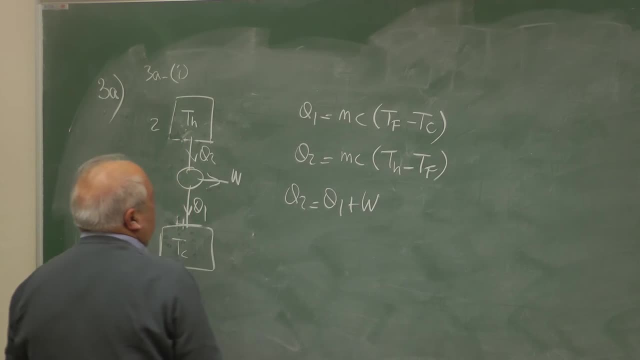 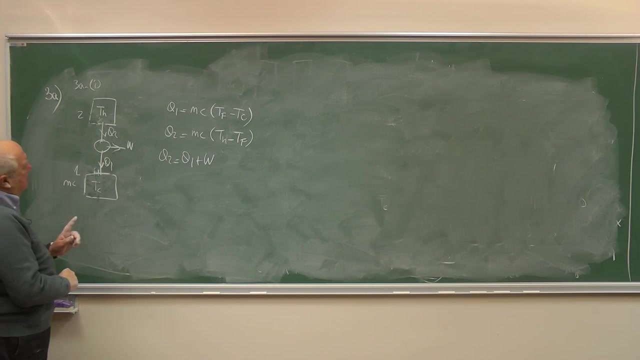 plus W, that's the conservation of energy. all right, that's the. but you see, TF is not known now, because we have three equations. but TF is not known, W is not no, so the we handle the head. we can get a handle on this problem by looking at the entropy, because it's a reversible. 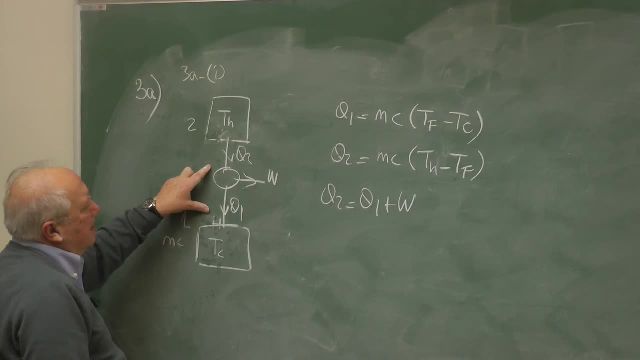 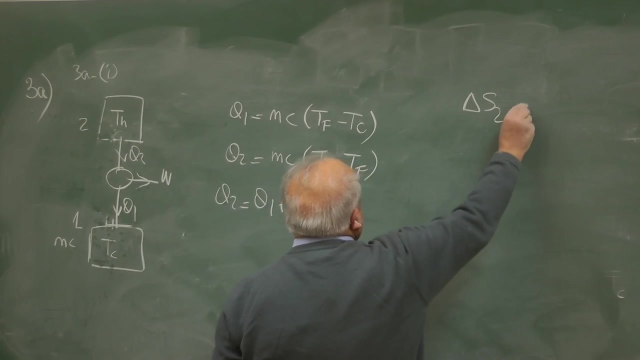 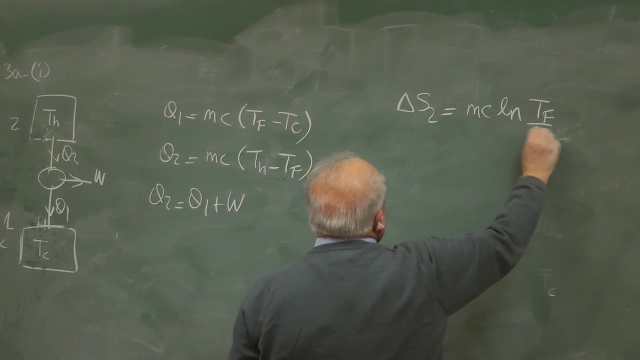 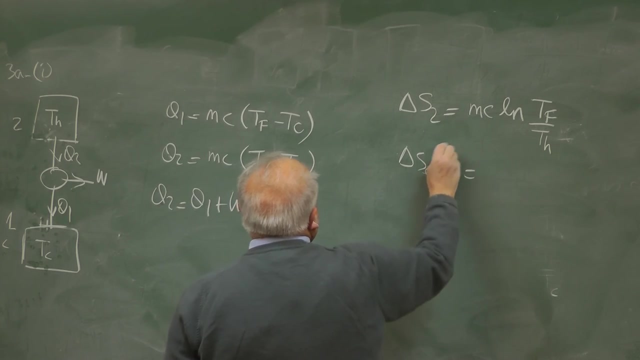 engine at the end of the day. at the end of the day it's a reversible engine and if you of the cycle, total entropy will be 0. so Delta is 2 is m C log T f over initial th Delta s engine. but because this was a cycle it is 0. Delta s 1 is m C log T f. 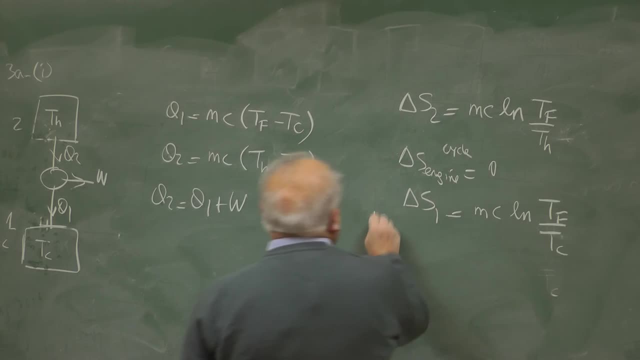 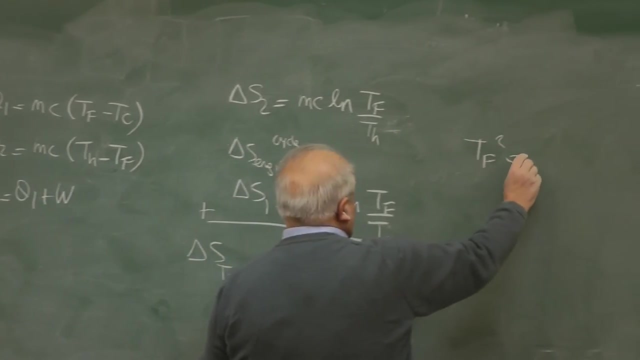 over TC. we add them up: Delta s total. now this must be 0 you, because it's a reversible cycle and remember the Clausius theorem. therefore this is equal to m C. if you just add them up, this is the log of T f square over th TC. now, if it is 0, this must be logo 1, so T f square is th TC over. 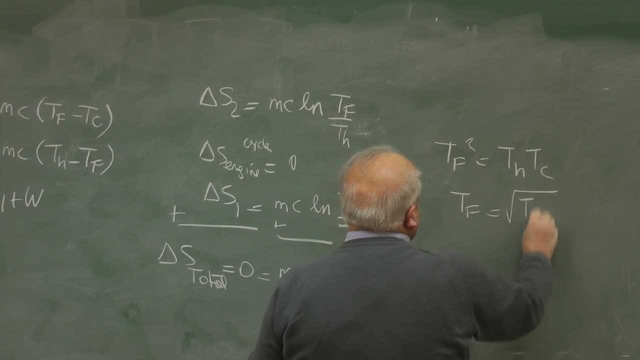 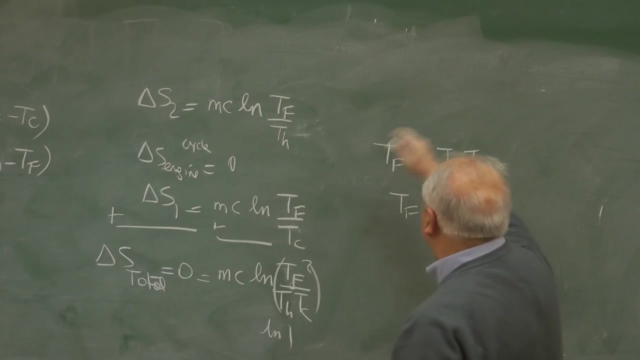 Wakthad right soup. also, this is equal to log T, odd success, or T f plus plus z, and this is equal to negative 3 T f or T f is equal to root th TC. now, this is difference from the final temperature of the irreversible process, T F. 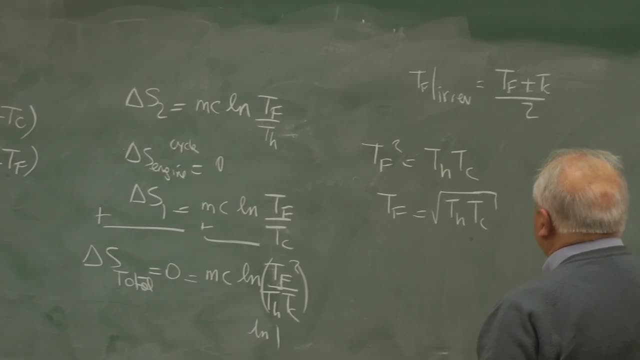 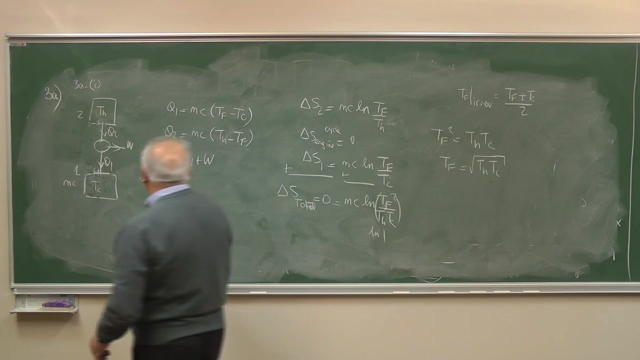 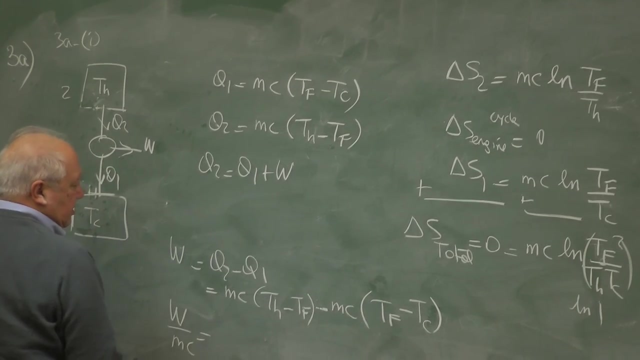 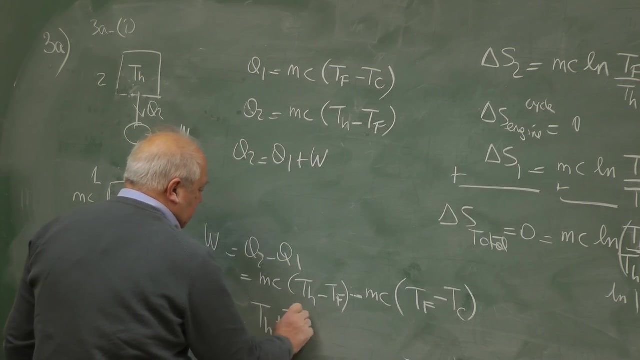 irreversible was the arithmetic mean T, F plus TC over 2. this is that okay and is: W is Q2 minus Q1, that is MC, TH minus TF minus MC, TF minus TC or W over MC is equal to TH plus TC minus 2 TF.